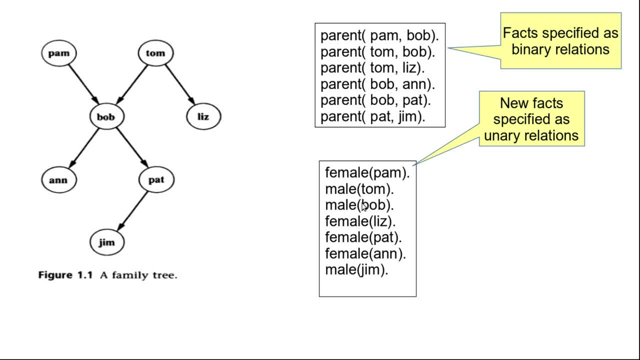 our unary relations. Instead, here we have two different relations. One is female, the other is male. Instead we can use only one relation, which the name may be gender, but have it as a binary relation. So here we say that gender of Pam is feminine, gender of Tom is masculine, and so on. 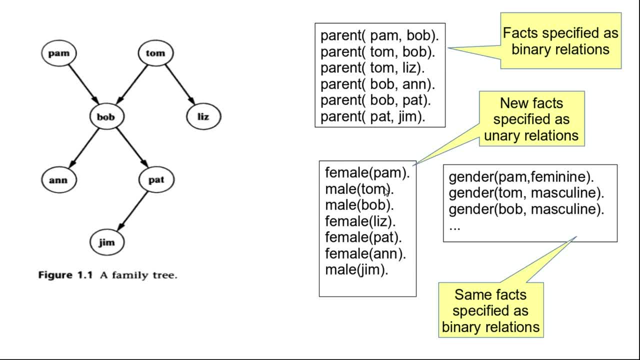 So here we have two different relations, but the relations are unary relations, But here we have only one relation gender. We do not have two separate relations, male and female, but we have only one relation gender, But the relations are binary relations. 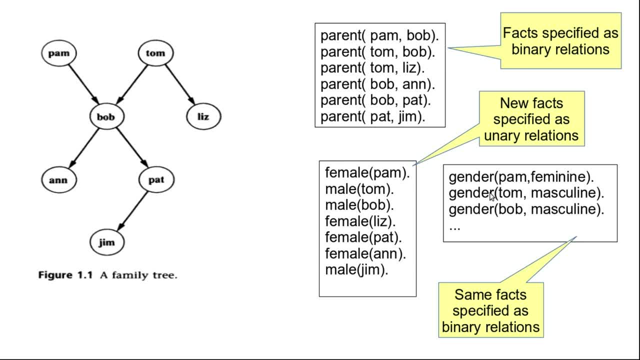 So to capture the gender information, we add new fact to our program. Now let us continue and let us see what about. we want to represent the mother relation also, So we want to capture the information: who is the mother of whom? 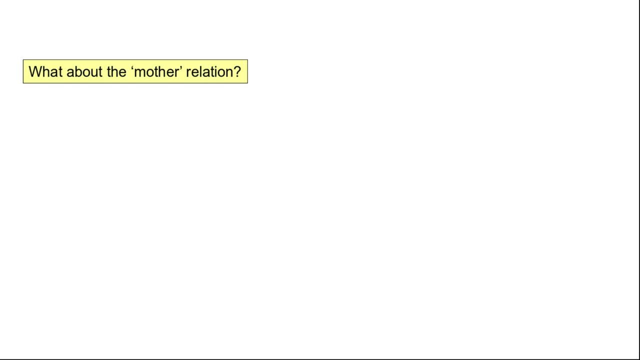 One way to capture this relation is to add new fact. So one way to capture this relation is to add new facts about the mother relation. So when we add new fact, it may be something like this: Pam is the mother of Bob, Pat is the mother of Zim, and so on. 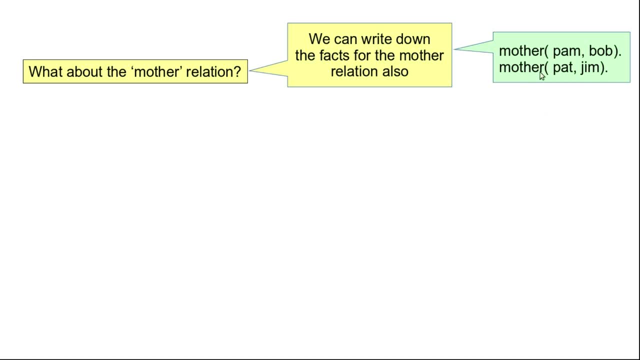 So we can add lot of fact here to capture the mother relation. However, there is a different approach Because the mother relation is unary. So we can add new facts about the mother relation. So we can add new facts about the mother relation. 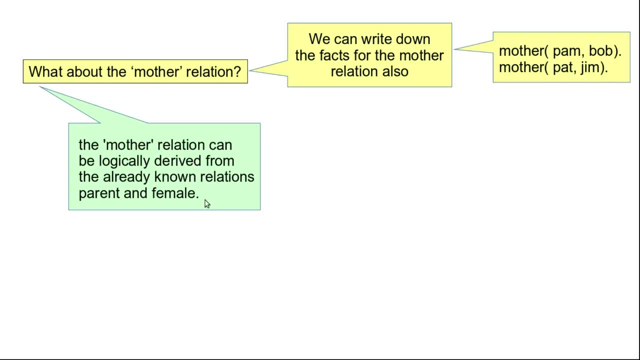 So it is written that the relation can be logically derived from already known relation. So if we know the parent relation and if we know the gender relation, we can automatically find out the mother information also. So using the parent and the gender information we can derive the mother relation also. 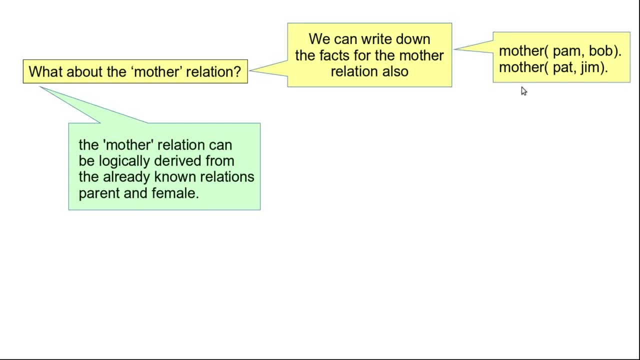 So it is not necessary to add new fact to our programs for all x and y. x is a mother of y if x is a parent of y and x is female. So we can say that x is a mother of y if, first of all, x has to be a parent of y. 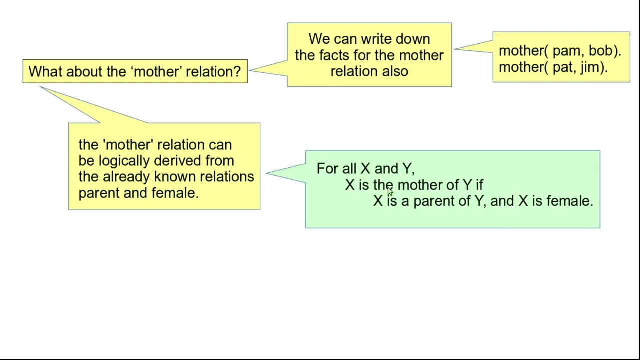 then only x can be mother of y, and x has to be female. So if this condition is satisfied, we can say that x is a mother of y. Now, in prologue, this particular logic can is represented as is shown here. So this is how we can represent this logic in prologue. 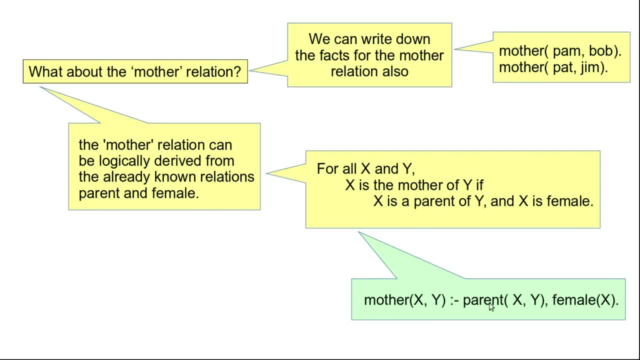 Mother x, y colon dash parent x, comma, y comma, female x. So this way of representing relations is called fact And this, the new method that I show here, this method of representing relation, is called rules. So fact, they are always true. 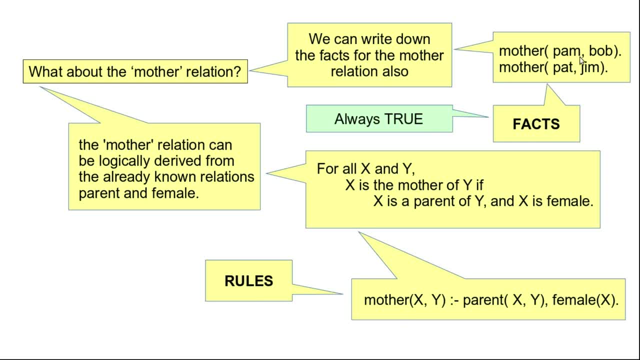 So if I say mother Pam comma Bob, then the fact that Pam is the mother of Bob is always true. However, in case of rules, the rules specify things that are true only if some condition is satisfied. So only if some condition is satisfied, this part will become true. So this is how rules work. 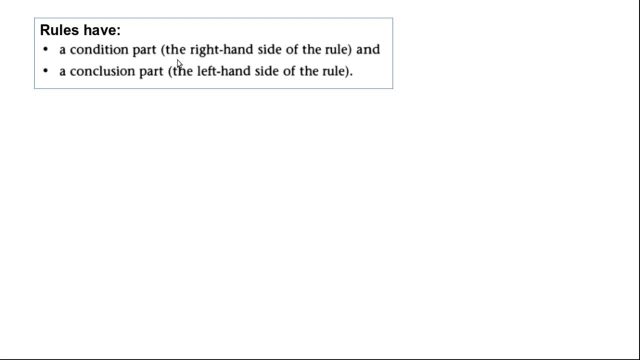 To continue further. so rules have a condition part, which is on the right-hand side of the rule, and a conclusion part, which is on the left-hand side of the rule. So on the right-hand side, this is the condition part. 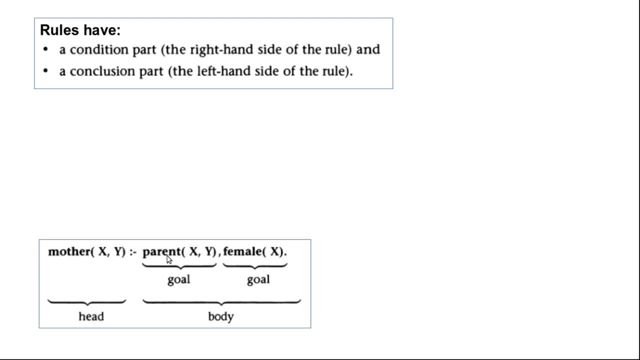 Parent x comma y, comma female x. So this constitutes the condition. And what is on the left side? Mother x comma y. This is the conclusion part. Um, the conclusion part is also called the head of the clause. so this is the head of the clause. and what is there under the 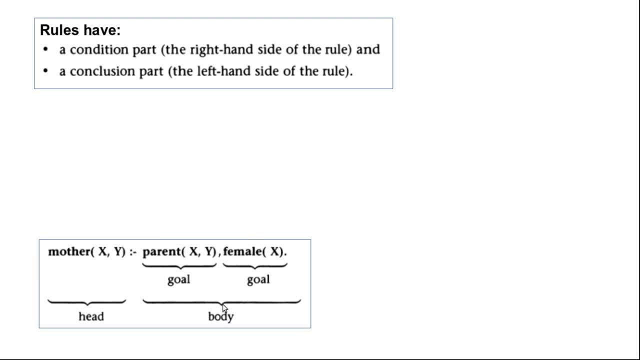 condition part. the condition part is also called the body of the clause. so in this case, in our body, we have multiple goals. one goal is parent X, comma Y. X has to be a parent of Y. the other thing is X has to be female. so so each of them is. 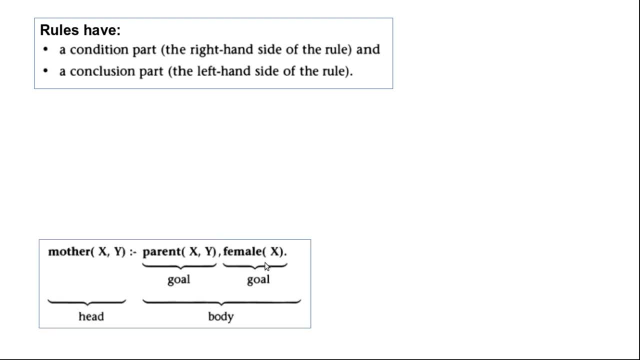 a goal, and this comma, comma means conjunction, the end operation. so for this body to be true, each of the goal has to be true. so this body part will be true only if parent X, comma Y is true and female X is true, only when both the goal is. 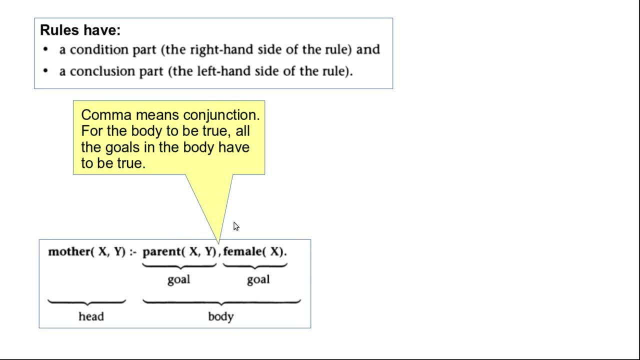 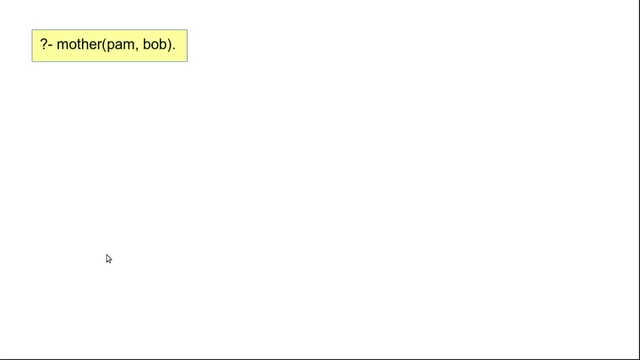 true, then only the body will become true. and if the body becomes true, the conclusion will become true. so if the body is true, then we can say that we can conclude that mother X is the mother of y. so now, continuing with that, after we represent the rule in our program, now we 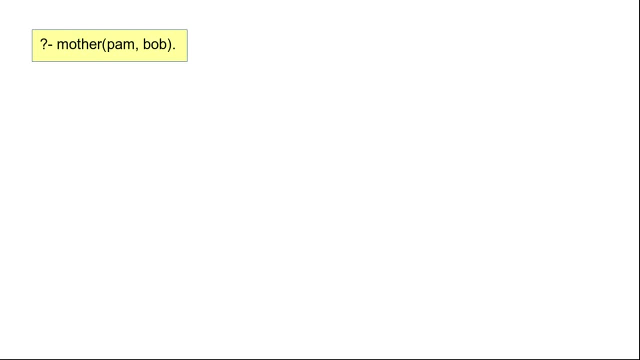 can ask queries to Prologue, queries like whether lifestyle meaningless宅 W. alors Pam is the mother of Bob or not. So we can ask this question to prologue Now we know that we don't have any fact. The only fact that we have in our program is the parent relation and male and female relation. 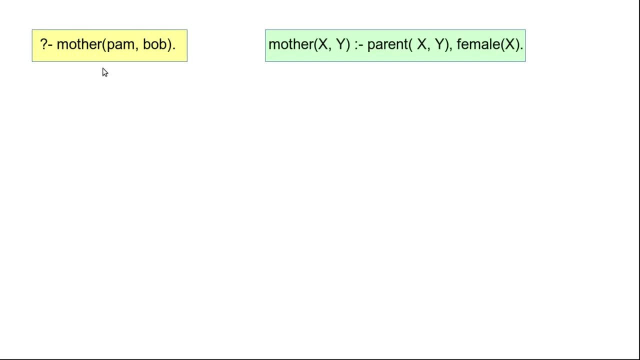 So these are the only fact that we have in the program. We don't have the mother relation as a fact. We have the mother relation only as a rule. So if I ask this question to prologue, whether Pam is the mother of Bob or not, prologue cannot answer it based on fact, because the mother relation is not present there as a fact. 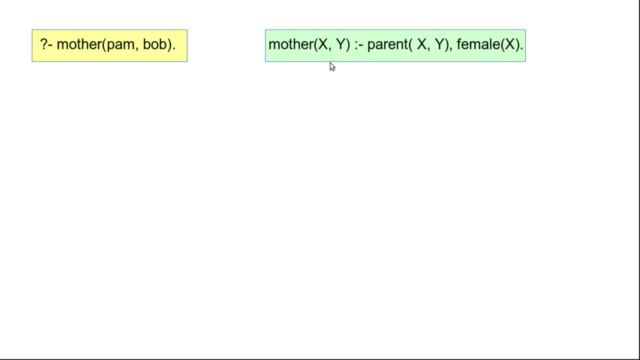 What we have is the rule. So now prologue will try to answer this question using this rule that we have in our program. Now, to use this rule, since we are asking about Pam and Bob, So these variables x and y has to be replaced with these objects Pam and Bob. So we say that we have to instantiate the variable. 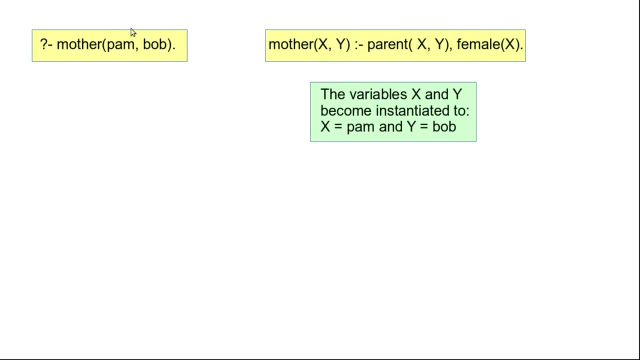 So x has to be instantiated, So x has to be instantiated to Pam and y has to be instantiated to Bob. Then from this rule we will get, after instantiation, this rule. We will get the rule that Pam is the mother of Bob only if Pam is the parent of Bob and Pam is female. So after instantiation of the variables, this is what we get. 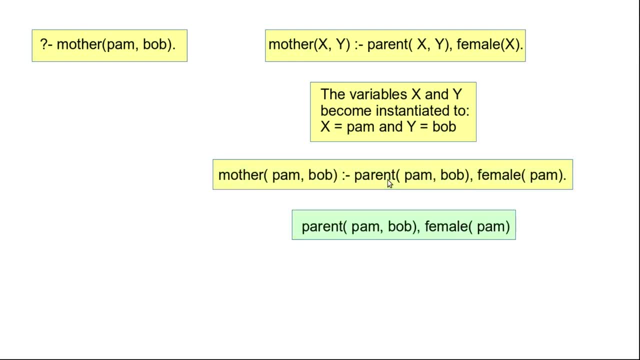 And now? So we have to answer this question: whether this part is true or not. Pam is the mother of Bob. Whether this part, the conclusion part, This is the conclusion part, For the conclusion part is to determine whether the conclusion is true or not. we have to determine whether the body is true or not. Now, what is the body? Body is Pam is the parent of Bob and Pam is female. So this is the conclusion part. 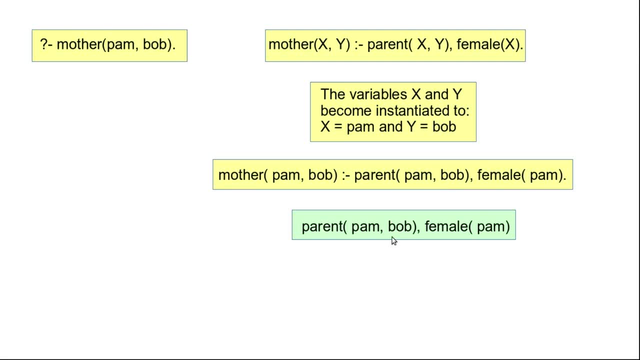 So this is the body of the rule. So now we have to determine whether this body is true or not. And to determine whether this body is true or not, we have to look at each of the goal. We have to first find out whether Pam is the parent of Bob or not, And then we have to find out whether Pam is female or not. However. so the initial goal of determining if a mother, Pam, is the mother of Bob. 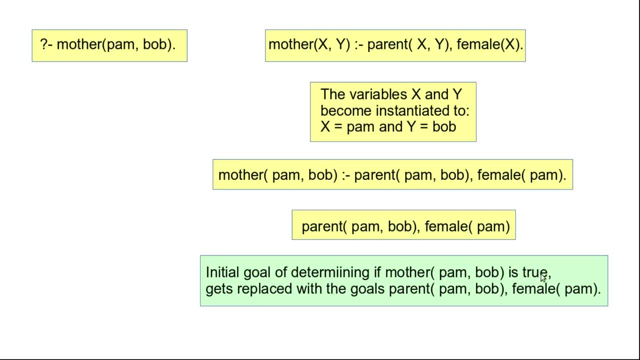 Whether this is true or not. That part gets replaced with the goals Whether Pam is the parent of Bob and Pam is female. Now, these two goals that we want to find out whether these two goals are true or not. This prologue will be easily able to determine whether these two goals is true or not, Because we already have fact related to the parents. 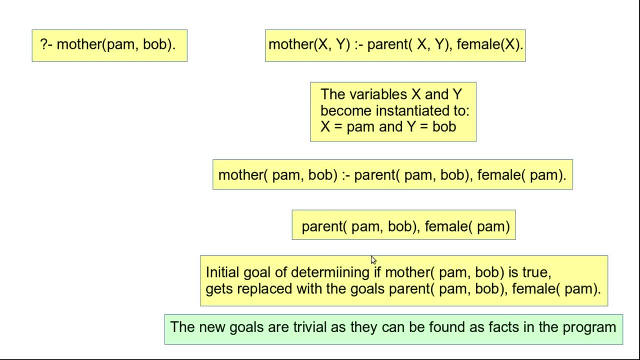 The parent relation and the female relation. So using those fact, I can find out whether these two goals are true or not, And actually we will be able to find out. this is true because in our program we have a fact which says that Pam is the parent of Bob, And in our program we also have a fact which says that Pam is a female. So based on those two fact, we can say that each of these two goals are true. 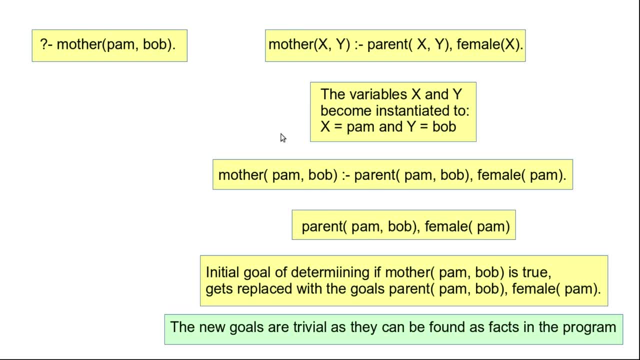 And hence, since both the goals are true, we can conclude that Pam is the mother of Bob. However, if any of this goal is false, if we don't have a fact which captures this goal, then that particular goal will be false, And if a goal becomes false, then the conclusion will also be false. But in this case, since we have, since both the goals will be true. 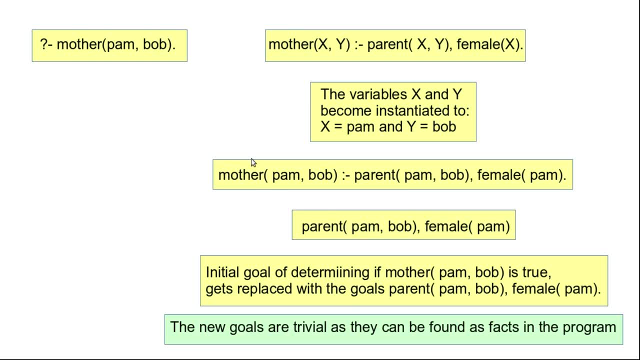 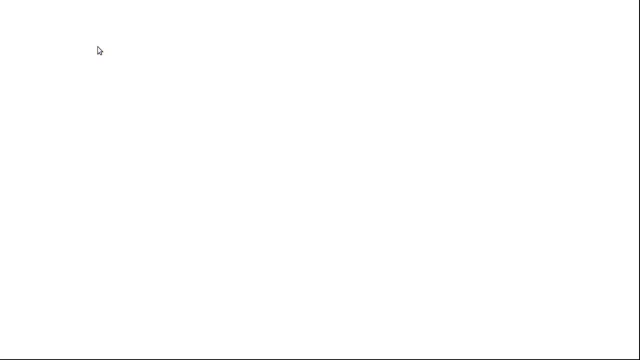 So our conclusion will be true and prologue will answer true for this question. That's all I have for today's class. Actually, we will run this program and see in execution. I'll show it in short. Okay, let me first show you executing the program. 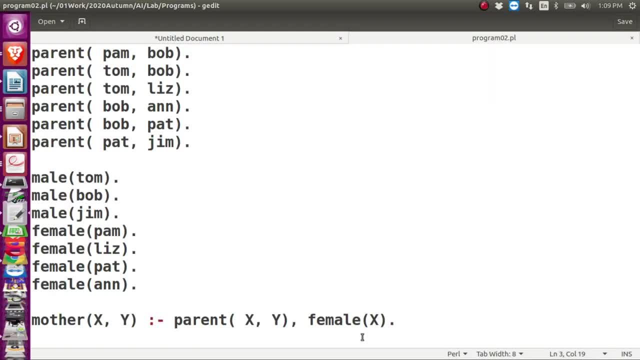 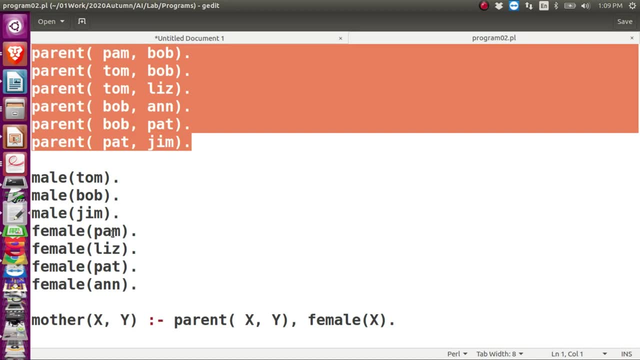 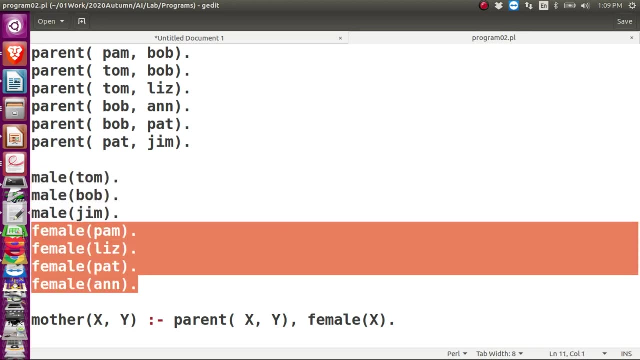 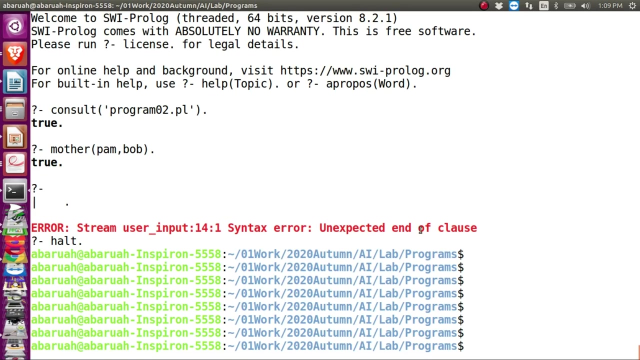 So first let me show you the program. This is the program that I have. As you can see, these are the fact: Parent relation fact. These are the fact related to the male relation And these are the fact related to the female relation, And this is the rule that I have in my program. So now, this is the program we have. Let me run SWI prologue. 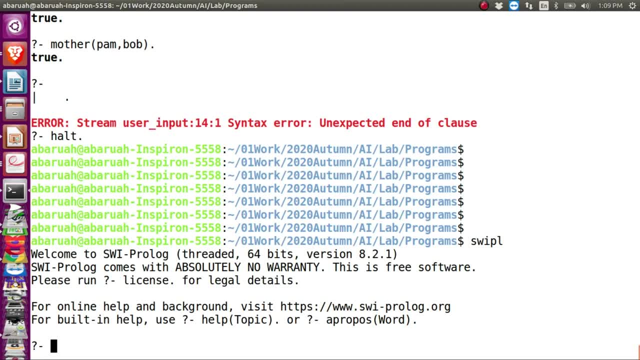 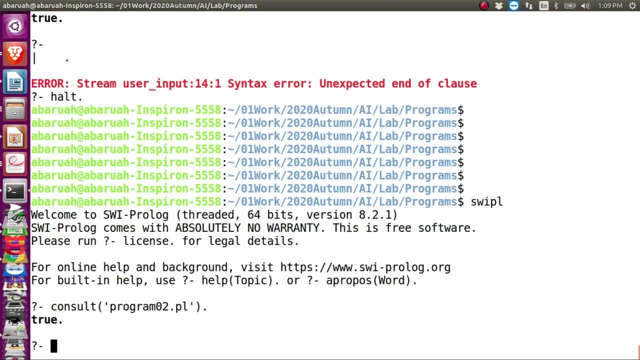 So let me start SWI prologue To consult. So I will consult program 02.. That's the name of my program, So let me load that program. So I have loaded it. So now I can ask the question related to the mother. So I can ask whether Pam is the mother of Bob or not. 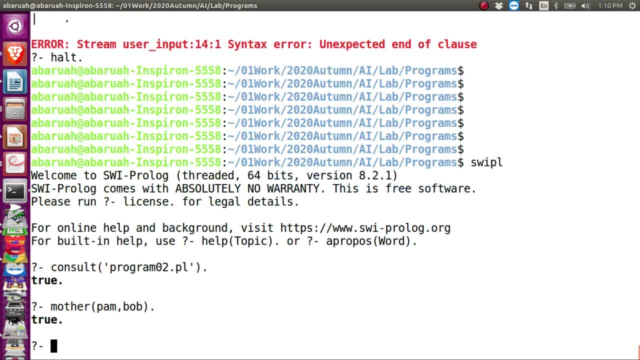 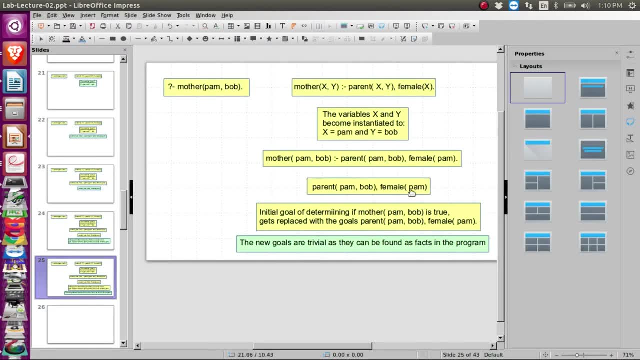 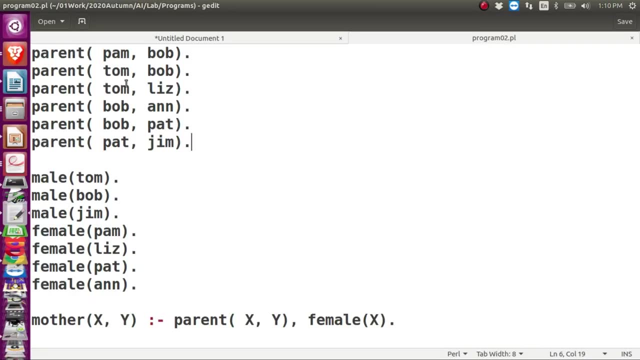 And if I ask that question Then it returns true, Because, as you can see, these are the two goals. we wanted to determine whether Pam is parent of Bob. Whether Pam is parent of Bob, Yeah, it is true, because we have a fact which says that Pam is a parent of Bob. And what was the second goal? The second goal was whether Pam is female or not, And I can find out from my program. 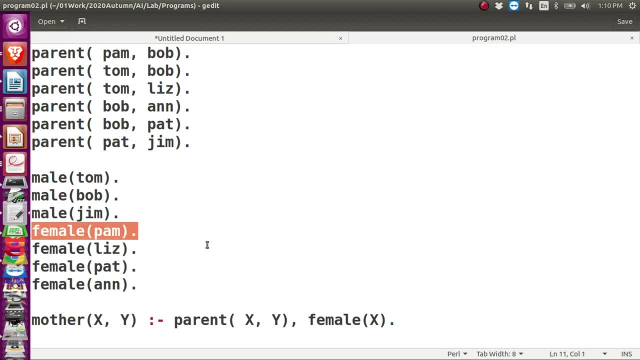 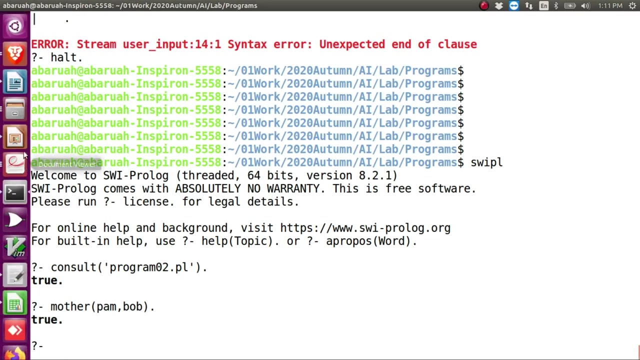 That Pam is female Hence, Since both the goals Are true based on the fact that are present, And hence my conclusion that Pam is the mother of Bob will also be true and prologue will, And prologue will answer true. Let us now try to give another query. 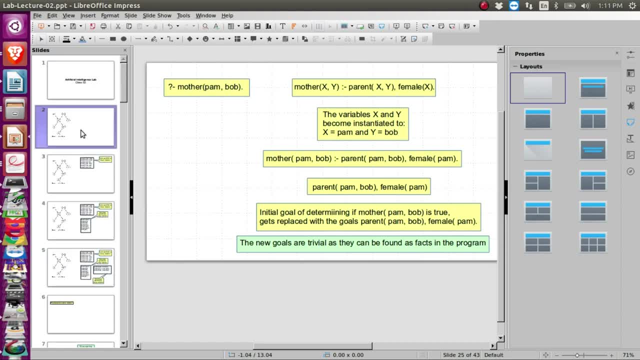 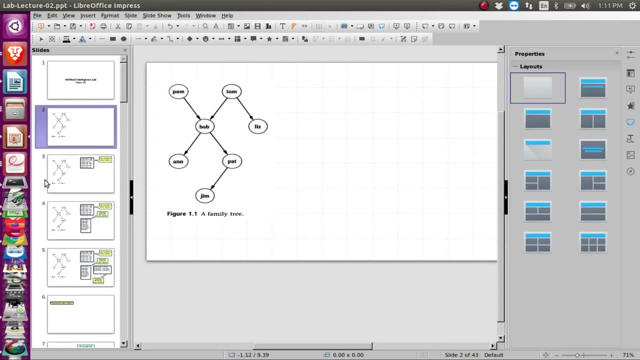 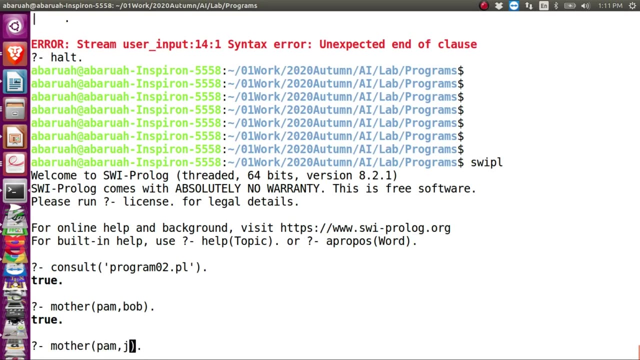 Let us look at our family tree. So let us ask whether Pam is the mother of Zim or not. So let me run that query: Pam is the mother of Zim. Now, when I ask this question, My goals will become. What will be my goals? 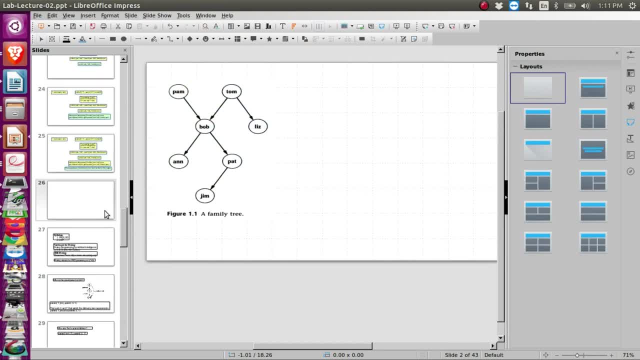 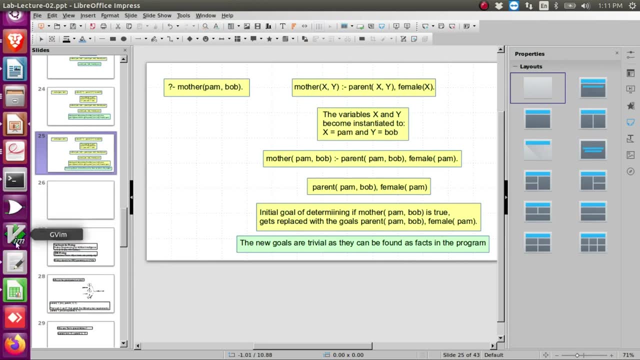 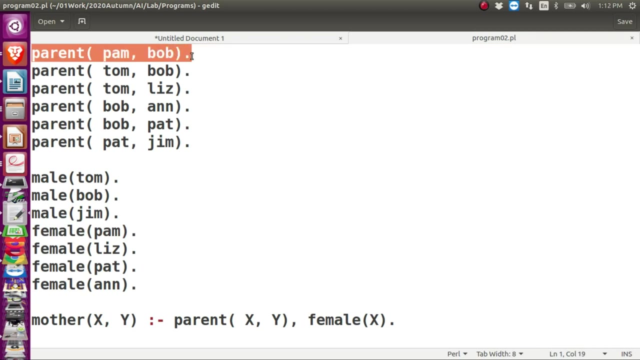 My goals. My goals will be: Parent Pam, comma Zim, Whether Pam is the parent of Zim or not. Now, there is no fact which says that Pam is the parent of Zim. We have fact which says Pat is the parent of Zim. 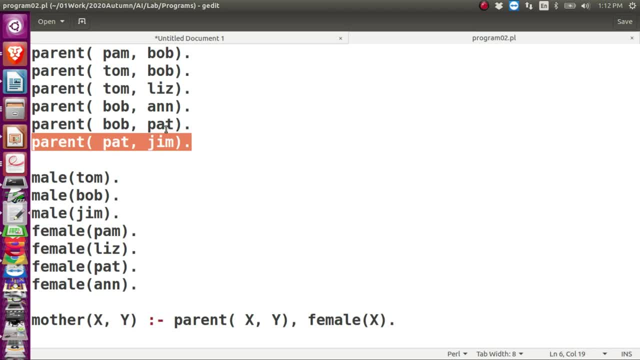 But we don't have any rule Which says that Pat is the Sorry, Pam is the parent of Zim, So that Particular goal will become false And which will make the body of the rule become false And hence the conclusion will be false. 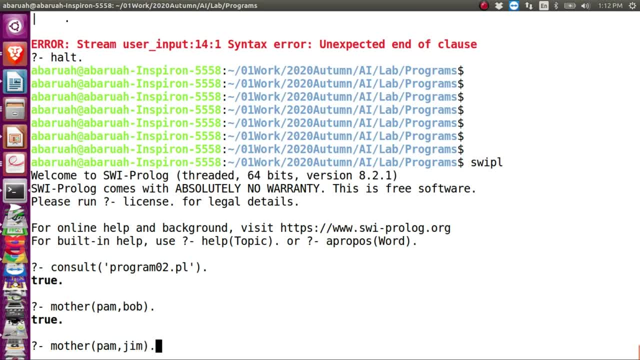 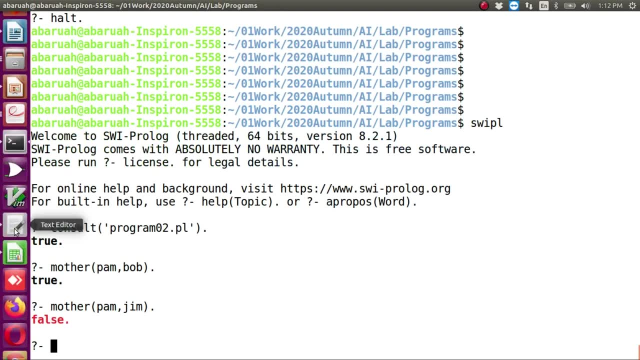 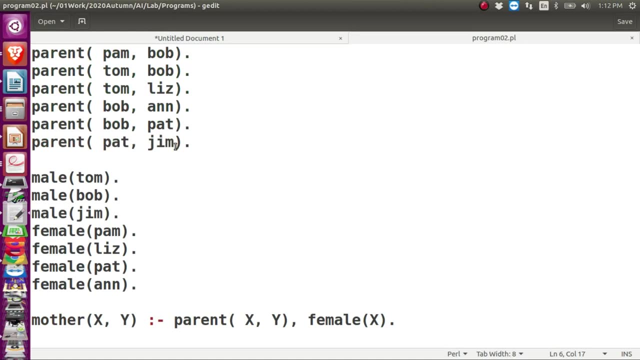 So prologue should return false for this question. Let us run it. Yes, it returns false. Similarly, However, if I ask whether Pat is the mother of Zim, Then we have this fact Present parent, And we also have the female Pat. 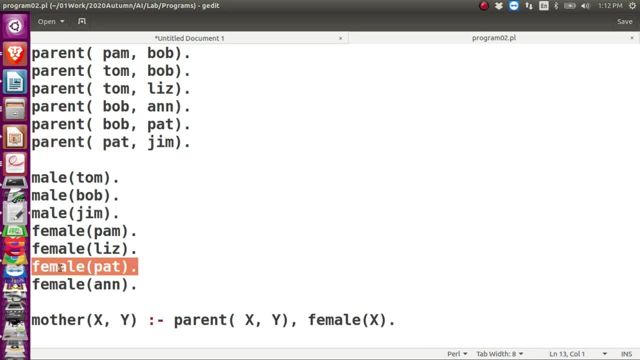 We have this fact also. So in this case, If I ask Whether Pat is the parent of, whether Pat is the mother of Zim For this query, Both the goals will be true. Hence, the conclusion that Pat is the mother of Zim will also be true. 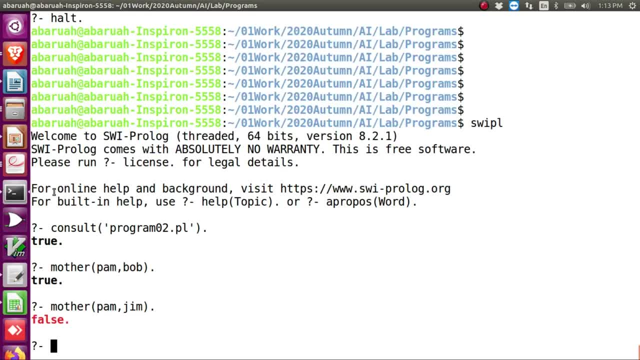